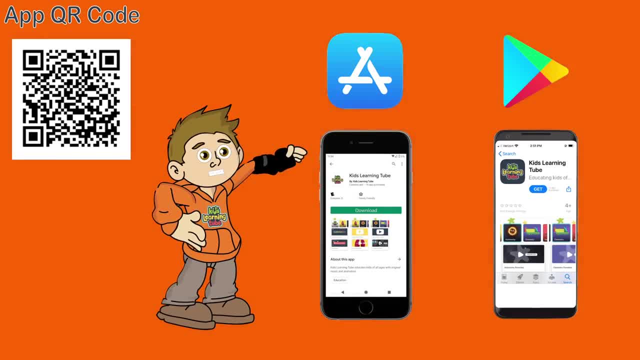 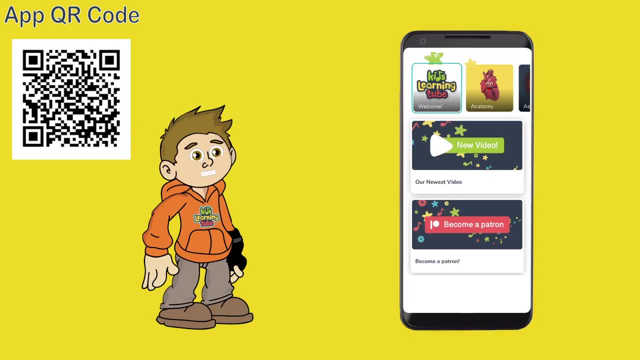 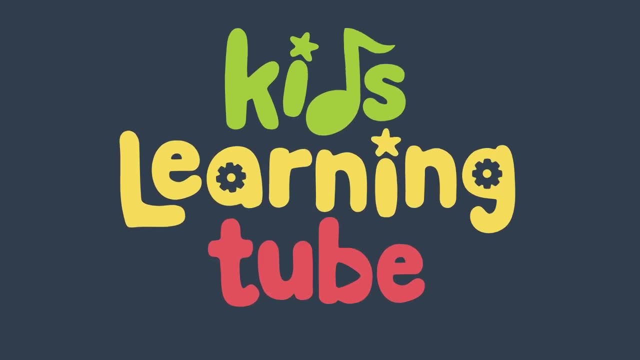 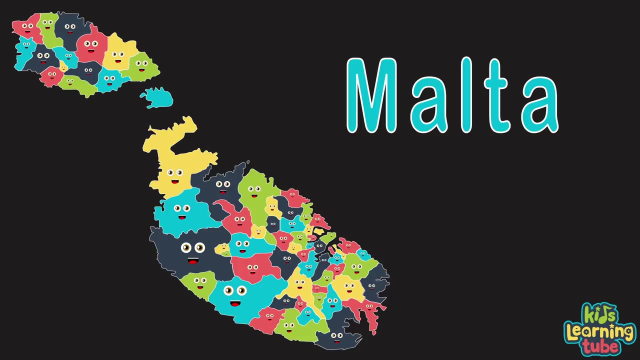 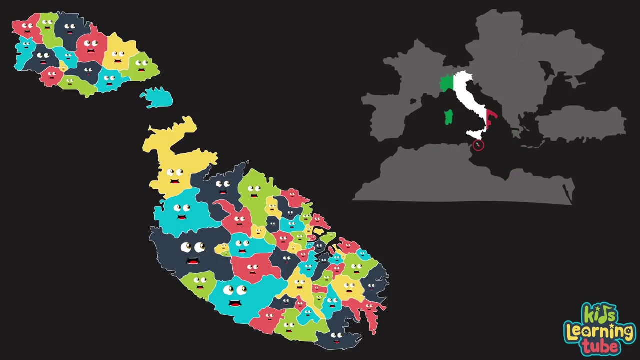 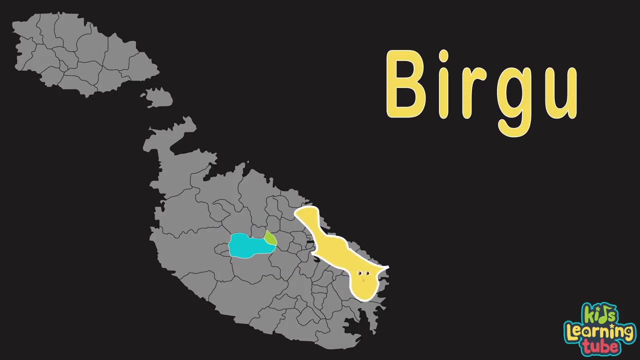 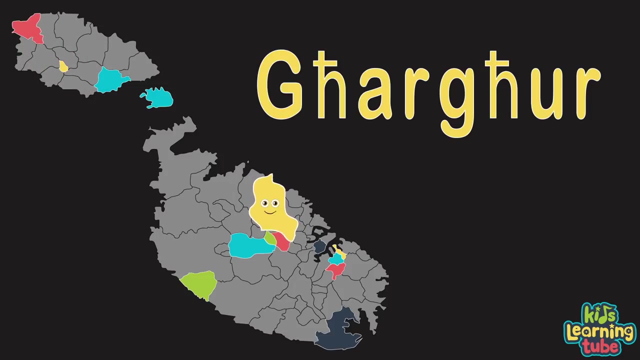 Search the Kids Learning Tube app on Apple and Android devices and download it today for a safe viewing experience while learning commercial free. We built this app just for you. We'll see you next time. See you on the Kids Learning Tube app. I am a tard. This is Berdson Bergu's. what you see. Bergekarazan Berzenbucha, Kaspikwa Dengli. This is Ofgura. I am Floriana, and Fontana Einselem and Alf Gargul Asri. 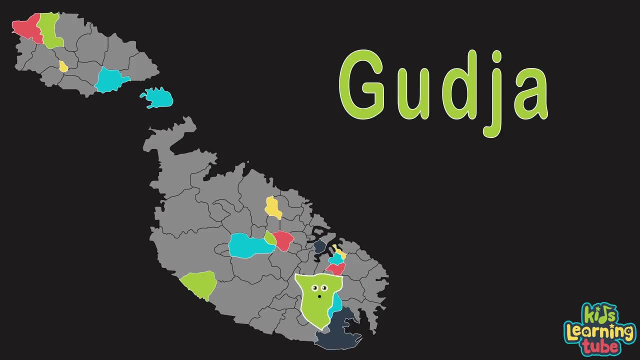 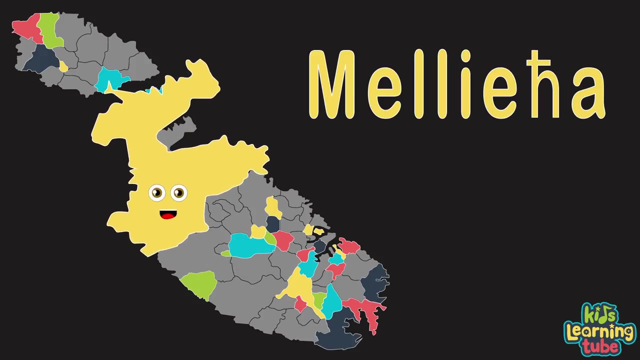 Asak Engugya. I'm Gzia Hamrun Liklin. Kalkara's fun, Kercham Kirkuk. I'm Lia And Lua, My name's Marza And Marza's Kala, Marza Shlok. I'm Dina Melia. 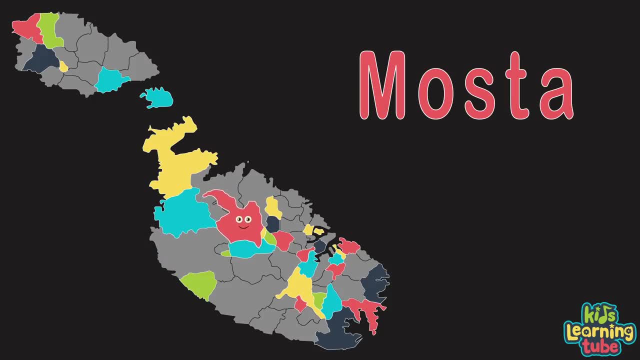 I'm Jar, I am Mosta, I'm Angba, I'm Sida And I'm Tarfa, Munchar Nadu, Nashar, Paola, Pembroke, Pieta And Ala Old me, Randy Safi. 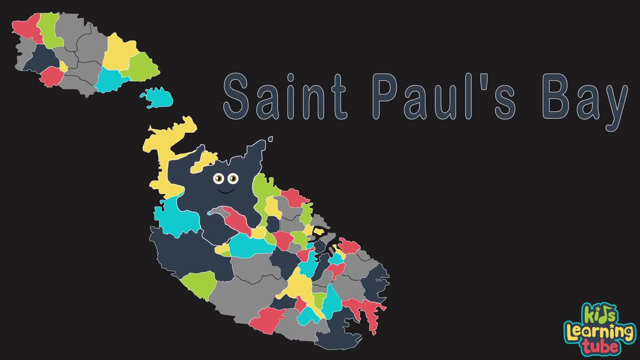 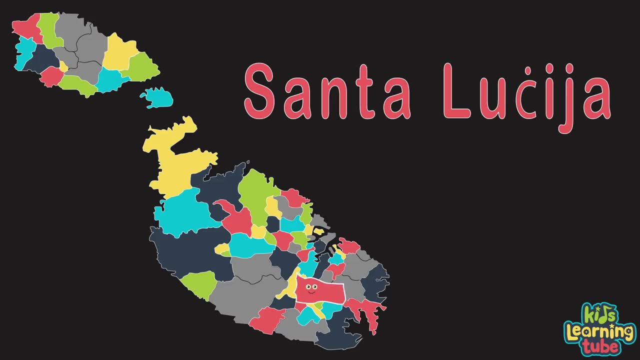 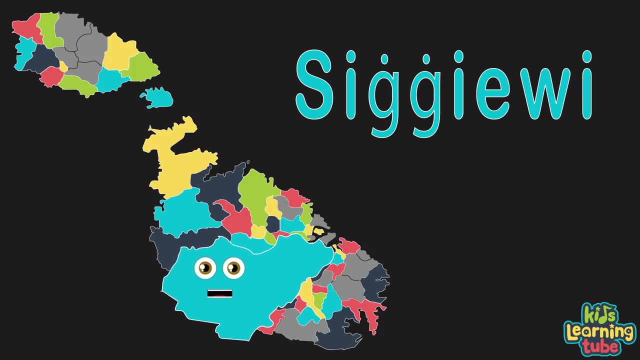 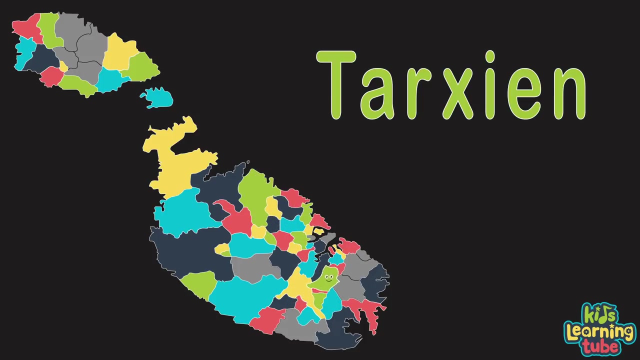 St Julian's In St Paul's Bay, San Juan, St Lawrence And Sanat Santa Lucia, Santa Vanya, Singlia, Sijui Slima, Sui Tarasin, I'm Valetta.